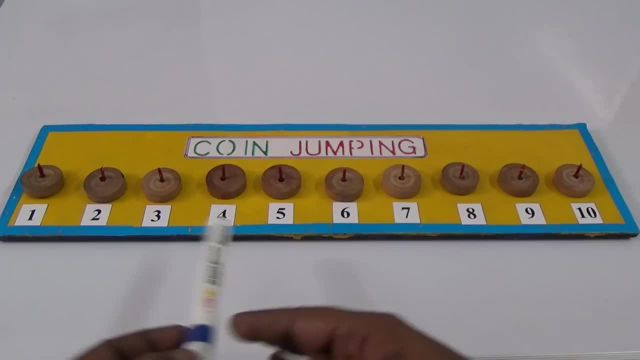 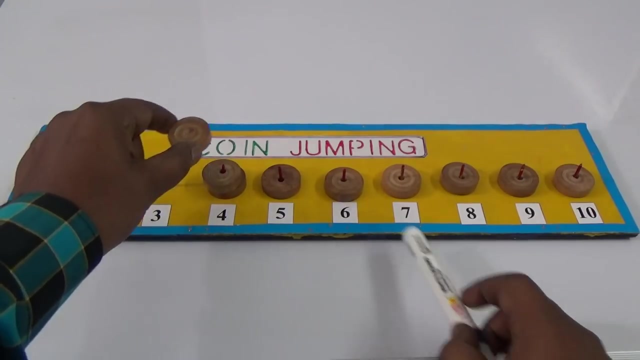 So in this puzzle it's a coin jumping. So if you observe here, total 1, 2, 3, 4, 5 and 6,, 7,, 8,, 9,, 10.. So 10 coins are there. So we need to use some rules and regulations to solve this puzzle. So first one is we need to take any coin and you can shift 2 coins when you want to place. For example, if you want to take this coin when you come out you're already 1, 2 are there, So you can come to only this place. So with minimum 5 steps, 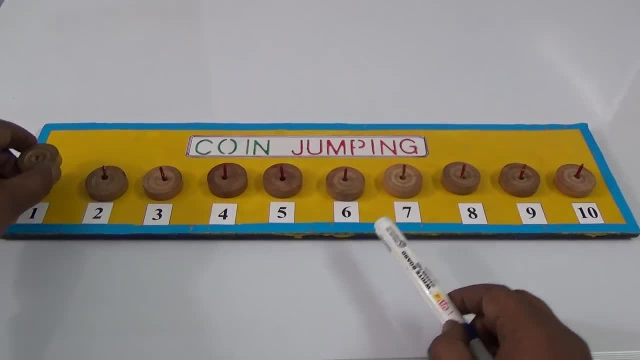 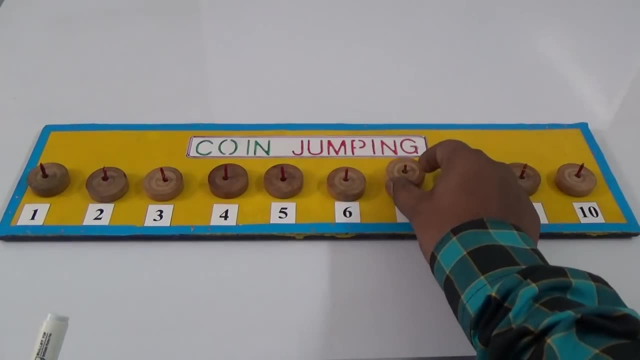 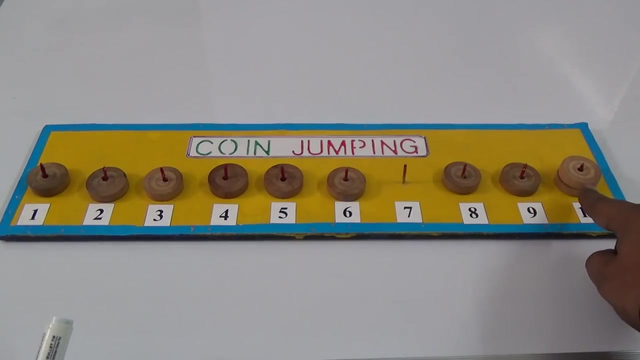 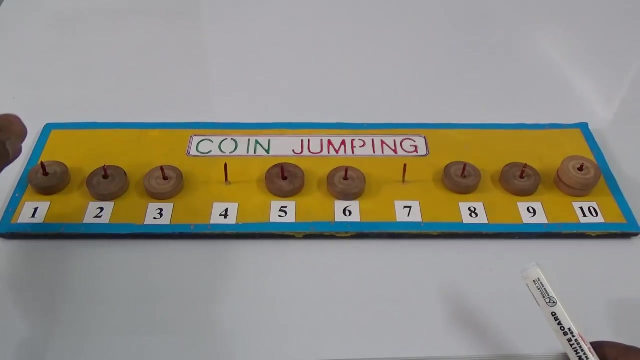 We need to take 2 bunches. That means every place. So alternate places should be 2, 2 coins. So for example, I'll try once here: From 7 to 10 I kept here, So it's jumped 2 coins. Now this is a 2 sets, It's a pair, That's it, So you can't take again more from this. Now, for example, if I can take this coin from 4 to 1, I can keep, Because it's all jumping 3 and 2.. Only 2 coins. it should jump. 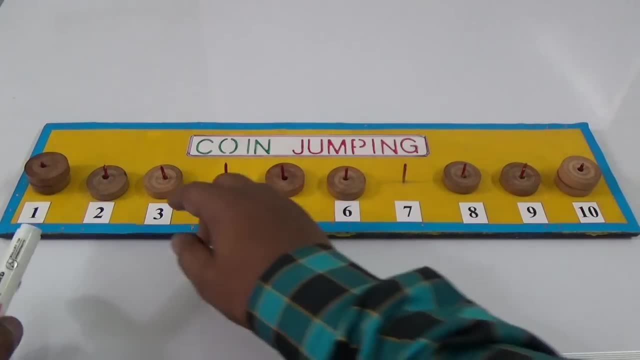 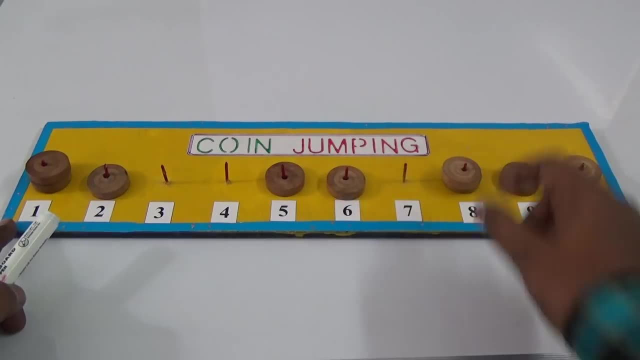 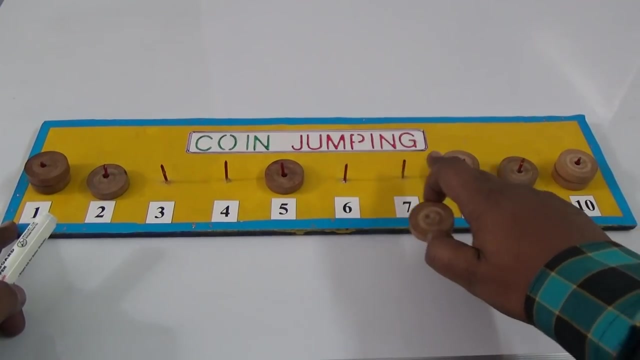 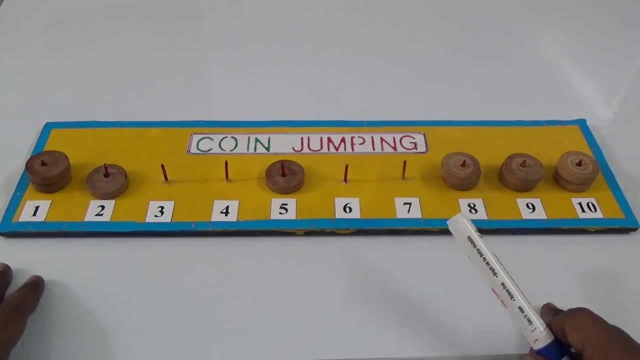 Now this one you can take, For example, if I want to take this: 3. When it's jumping, only 2 coins. What are the places? 1, 2 and next coin only should be placed Now, for example, this coin: if you take 6. 6, I can jump In this. 2 are there. So by 2 jumping it should be here Now. there's no chance. This is 1 extra left to 1 extra left, But we need to make alternate places. there should be 2, 2.. 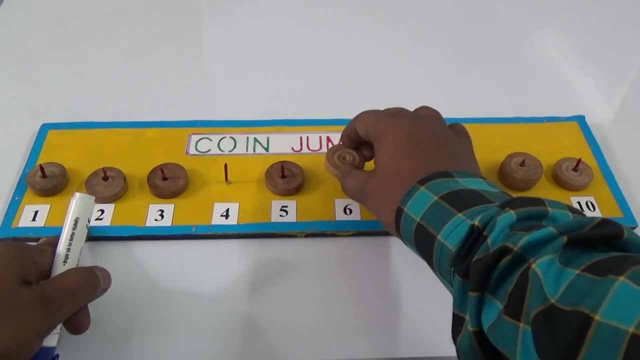 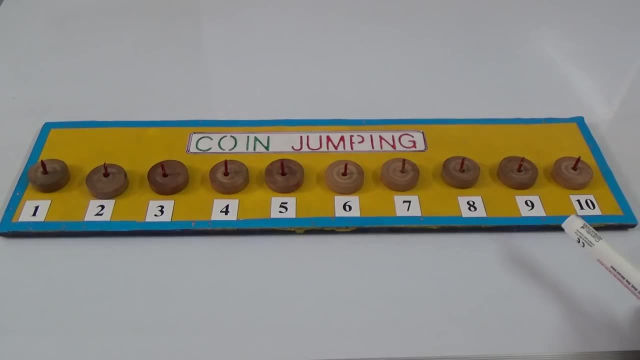 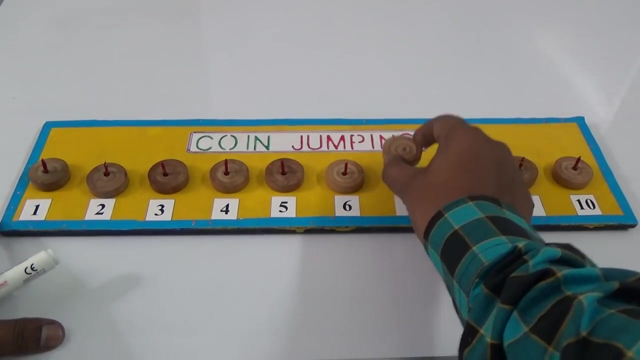 We need to jump only 2 coins And with the minimum steps, Only 5 steps. you need to make 2, 2 pair. So every alternate place, 2, 2 pair you should make. So let me solve the solution here once now. See here: First I'm taking 7.. Okay, this is one solution. You can take many also for this. And from 7 I'm keeping it number 10. Right, So 1, 2. 2 coins are jumped.